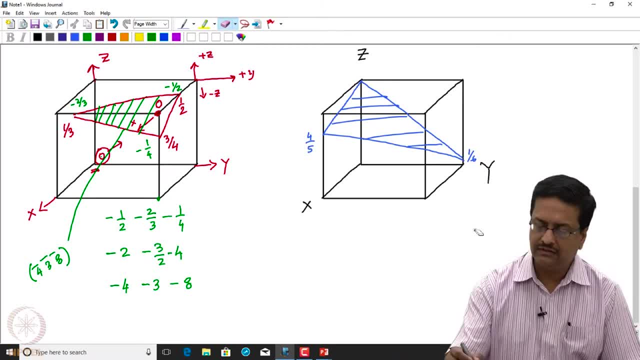 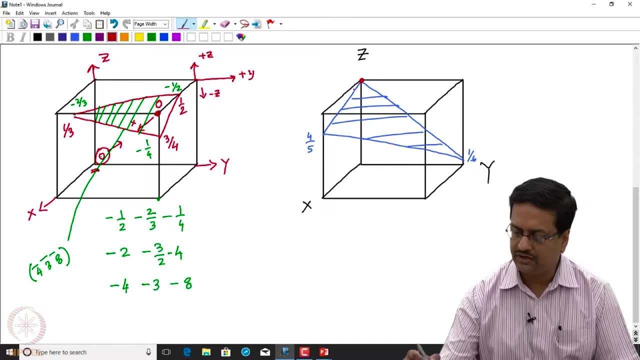 what we should do in this case. See what has happened- is when the line that we have drawn from the topmost point to this point- this is the line that is travelling along x- It has travelled one unit cell along x and it has come down from top by one fifth unit while travelling one unit. 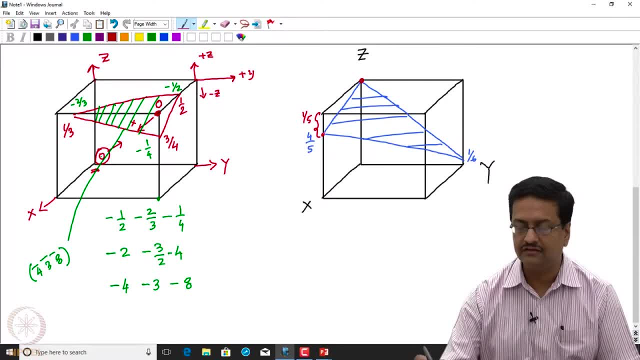 along x. So if it travels 5 such units on this side then this will go and meet the x axis. So on the side of y this has travelled one unit along y, but it has come down by 5 sixths along y. 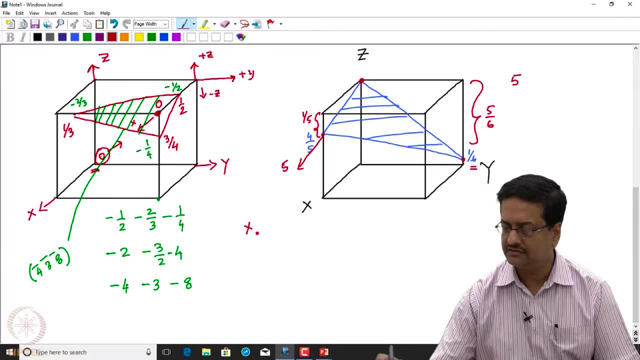 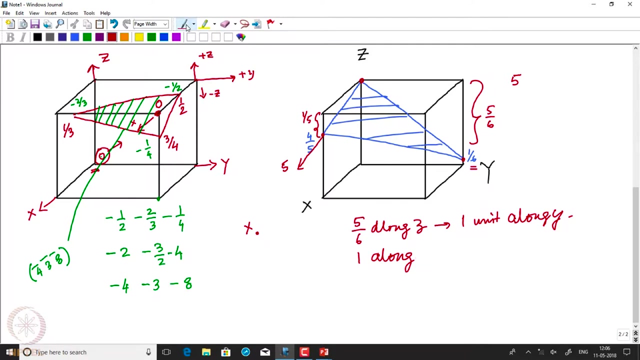 So if it has come down by five sixths along z, the line that we showed you was its z axis. Now, on the side of y, this has travelled one unit along z, but it has come down by 5 sixths unit along y at 1 along z will be travelled will be travelled: 1 along z will be travelled. 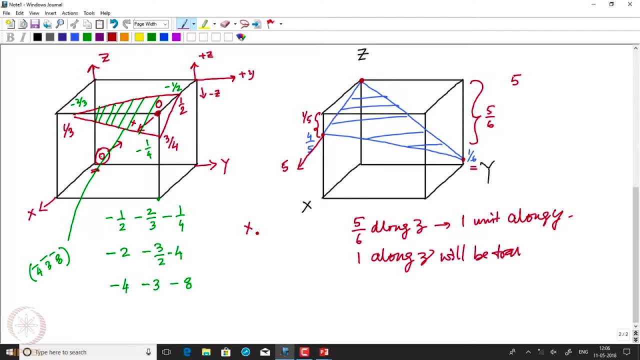 in sixth, fifth unit along y. So the y intercept will be 6 by 5 and from this point the intercept on z is 1.. So these are the actual intercepts. So the reciprocals will be 1 by 5, 5 by 6 and 1. then 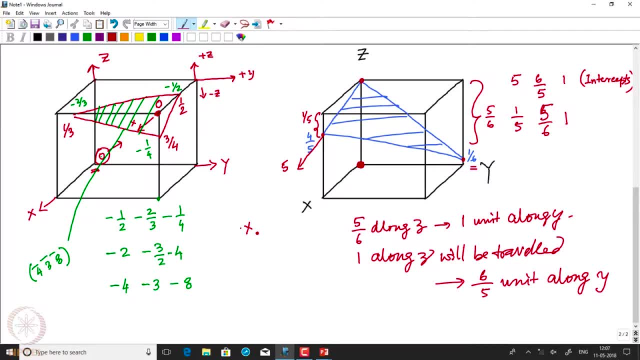 you clear fraction, So multiply by 30. So here you get 6, 25, 30. So the Miller indices for that particular plane becomes 6, 25, 30. This is to introduce that the Miller indices can be large, as large as we are writing, like 35, 25 and so on. So 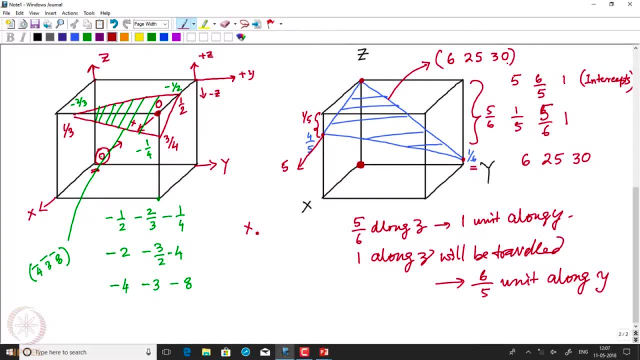 depending on how high the resolution data is, you can slice the unit cells into smaller and smaller and smaller fractions, and that is where we end up getting Miller indices for different planes, which are reasonably high. So I would like you to practise this Miller indices for next few days. 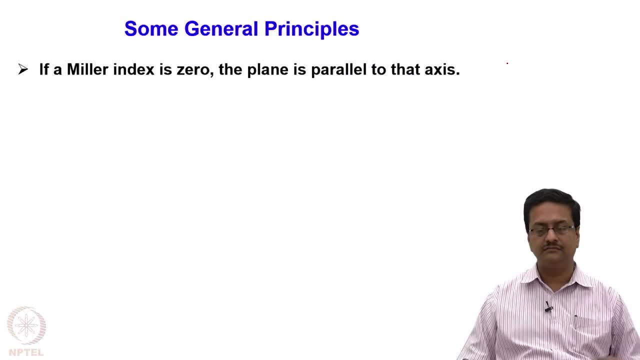 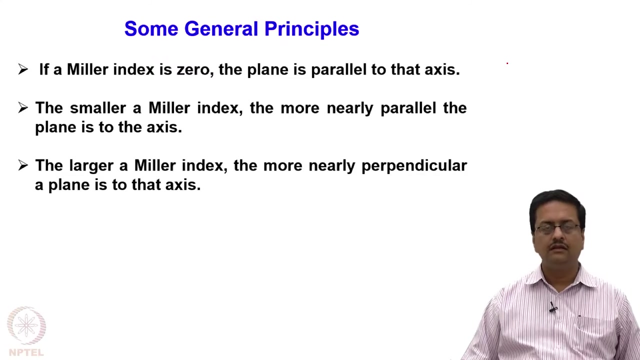 So we would like now to highlight some of the general principles, As we have already seen that if a Miller index is 0, the plane is parallel to that axis. The smaller the Miller index, the more nearly parallel the plane is to that particular axis. The larger 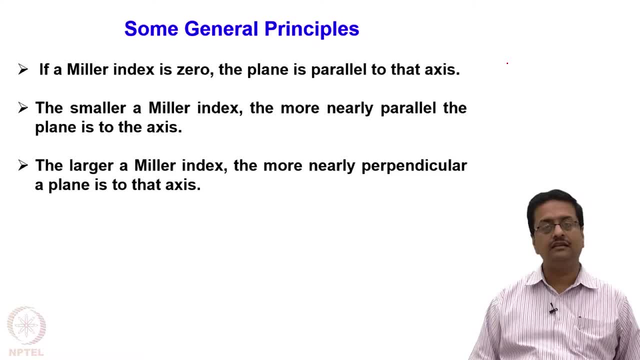 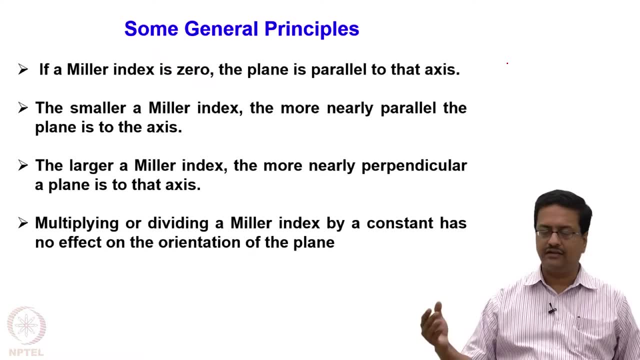 the Miller index, the more nearly perpendicular a plane is to that particular axis. Multiplying or dividing a Miller index by a constant has no effect on the orientation of the plane, but it indicates a parallel plane. Miller indices are almost always small for routine. 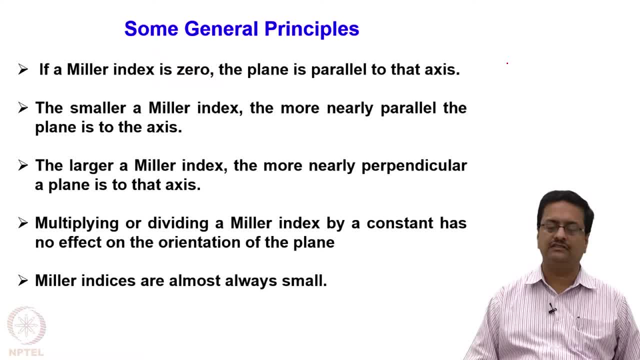 data because we are only worried looking at a very small fraction of the two things at a much higher angle, at which we collect the data For your homework, I would like you to draw different planes like 1 0 0, 2 0 0, 1 2 bar. 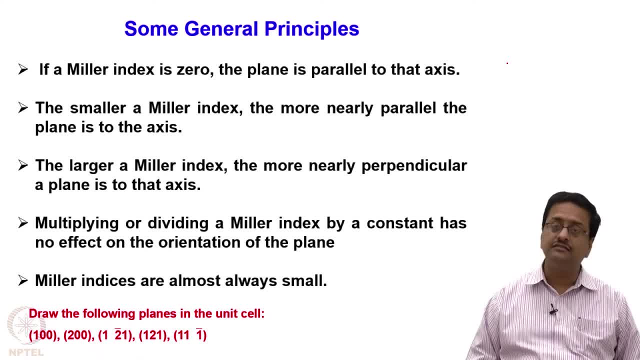 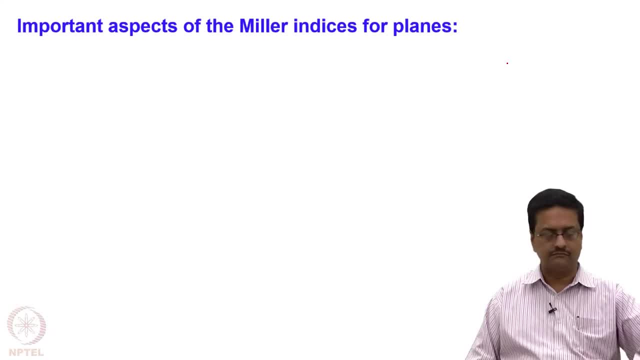 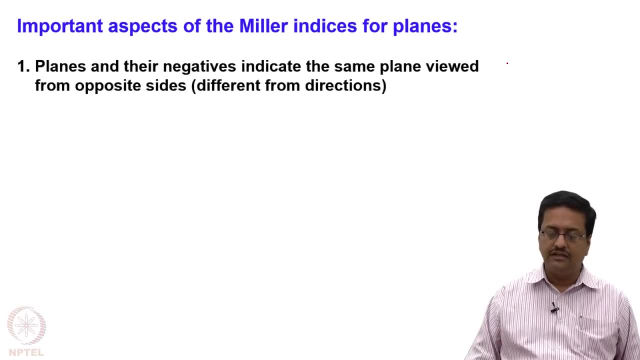 1, 2, 1, 2, 1, 1, 1 bar. kind of plane Practice: drawing these different planes within the unit cell. more points: Perseverance. Some important aspects of the Millerwal index: P Basil indices for planes: continues. the planes and their negatives indicate the same plane viewed. 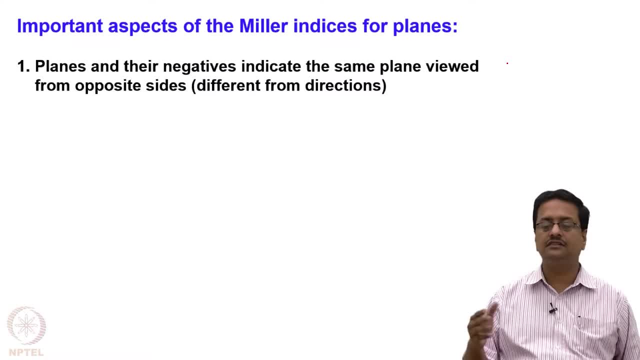 from opposite side or different. this is different for directions. So if you have a plane h k l and you are talking about h bar, k, bar l bar, you are looking at the same plane from two different directions, Whereas in case of crystallographic directions a plane h k l is opposite in direction. 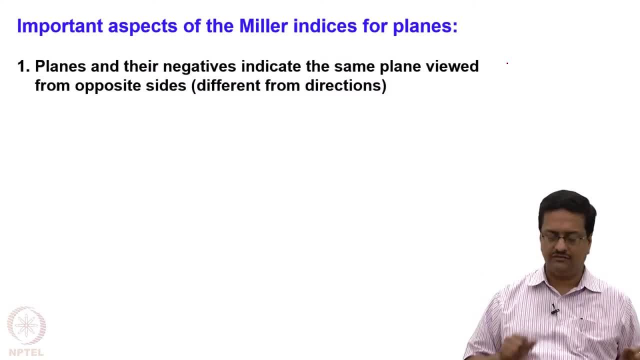 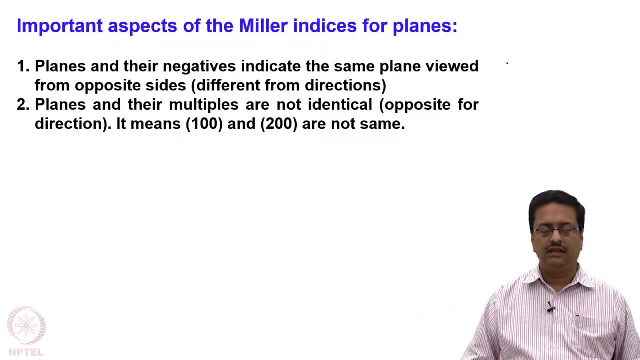 compared to a plane direction: h bar, k, bar, l bar. So there are two opposite directions. planes and their multiples are not identical. Again, this is opposite from that of directions, which means the plane 1 0 0 and 2 0 0 are not same, but in case of direction, the direction, 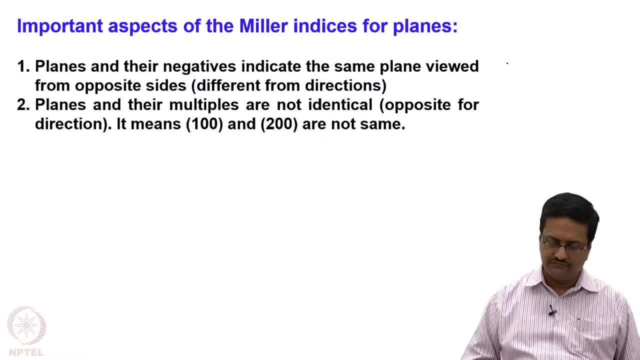 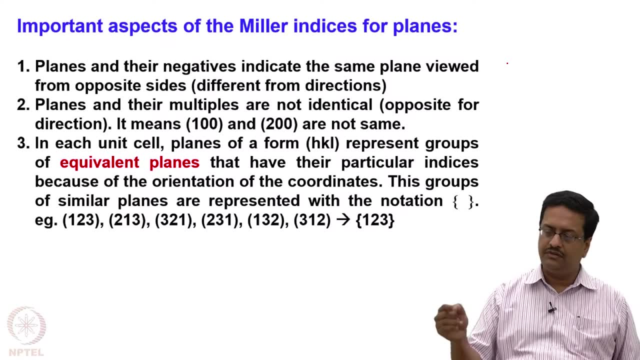 1 0 0 and 2 0 0 indicate the same direction In each unit cell. planes of a forcing form, Hkl, represent groups of equivalent planes that have their particular indices because of the orientation of the coordinates. These groups of similar planes are represented with the curly. 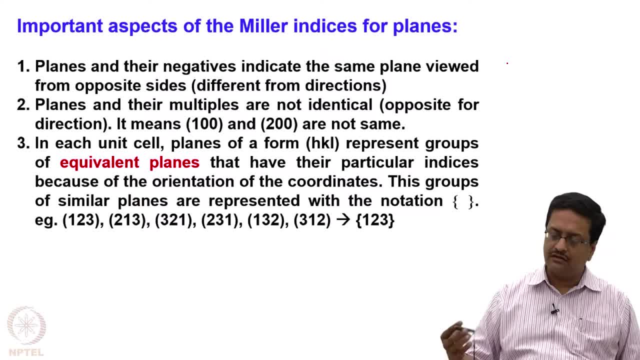 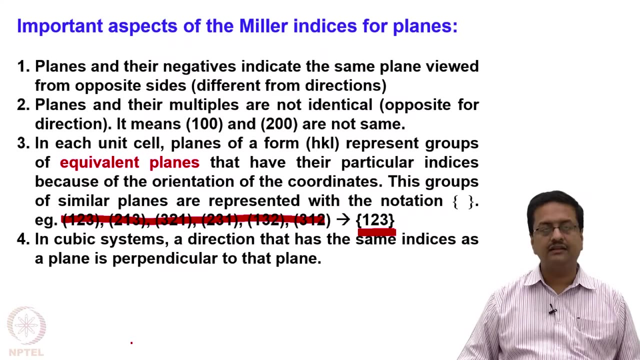 brackets. So these are called as family of planes, as we have already indicated. So these planes are highlighted as a family of equivalent planes 1,, 2, 3.. In cubic systems, the direction that has a direction that has the same indices as a plane is perpendicular to that particular plane. 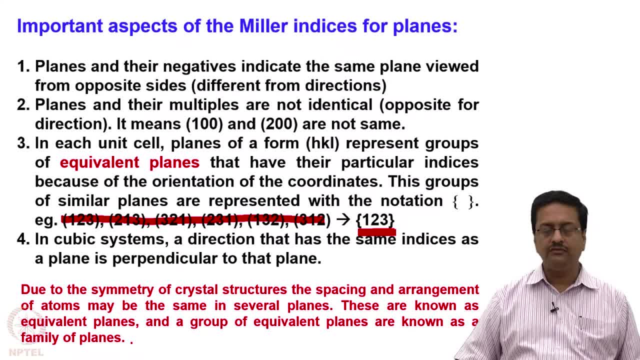 Due to the symmetry of the crystal structure, the spacing and arrangement of the atoms may be same in several planes. These are known as equivalent planes and the group of equivalent planes are known as family of planes. So to conclude this section, I am: 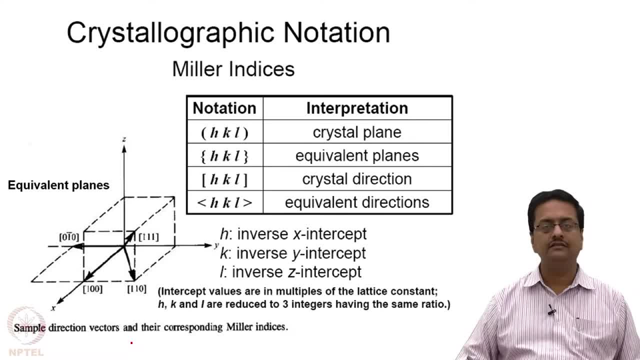 bringing this slide in- that when we try to write the Miller indices, when we write it usingب this sheet, first bracket, like h k l and we do not have any comma, it indicates a crystallographic plane. When we write h k l within the second bracket, as indicated here, we are talking about equivalent. 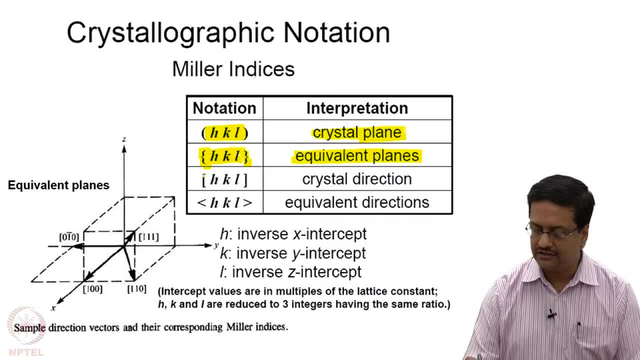 planes. When we are indicating the h k l within the third bracket or the square bracket, it indicates a crystal direction, and when we represent h k l within this greater than less than sign, they are called the equivalent directions. So with this we will. 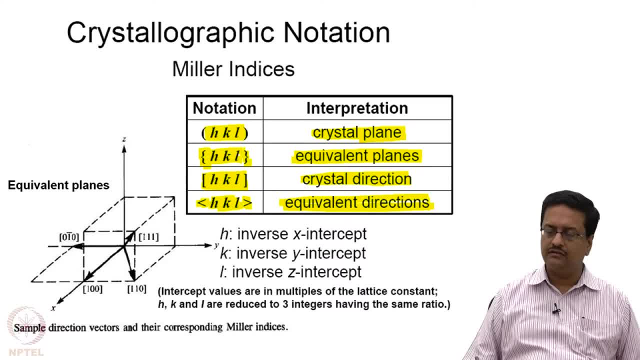 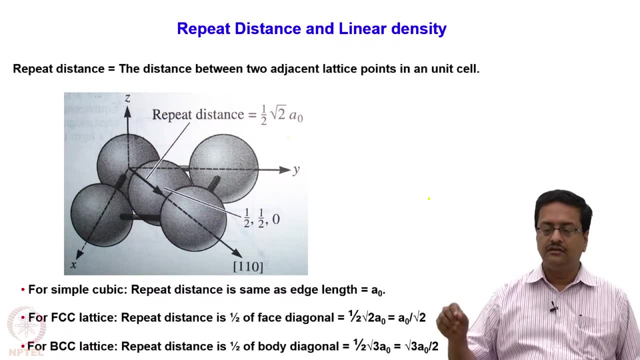 conclude the part where we needed to know the Miller indices for different set of planes in different crystallographic systems. So now we would like to concentrate on a different topic, where we would like to see what are repeat distances and linear density. A repeat distance: 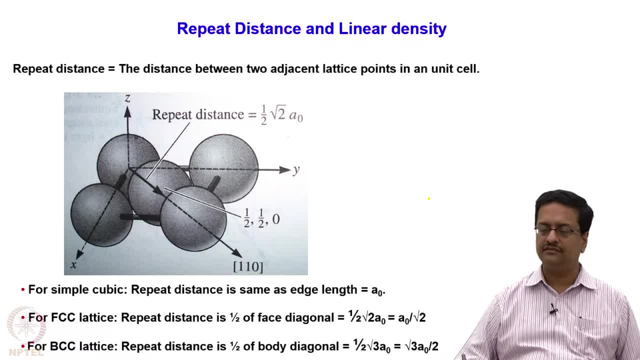 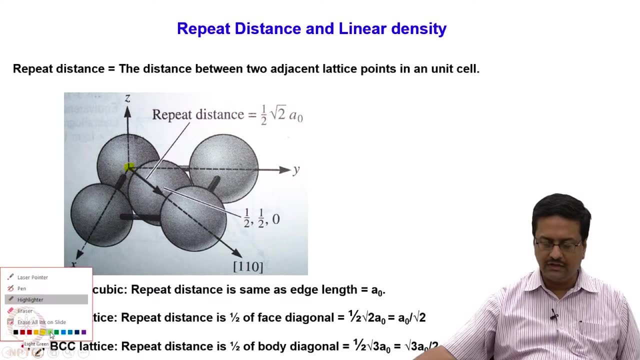 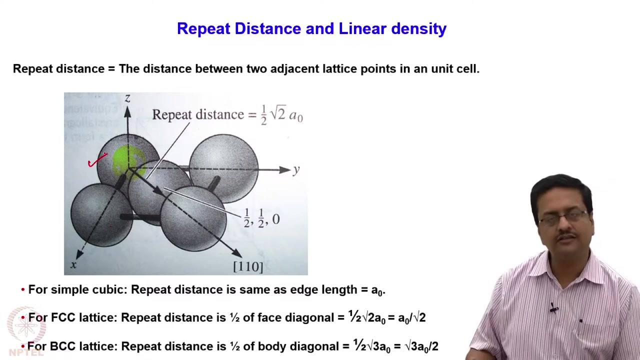 means the distance between the two adjacent lattice points in the unit cell. So in case of a face centered lattice, what we have is an atom at the center of the face and an atom at the. in the figure here what we see is that you have one atom at the center of one atom at the. 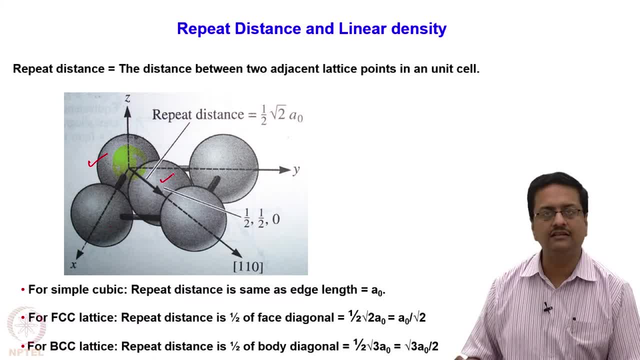 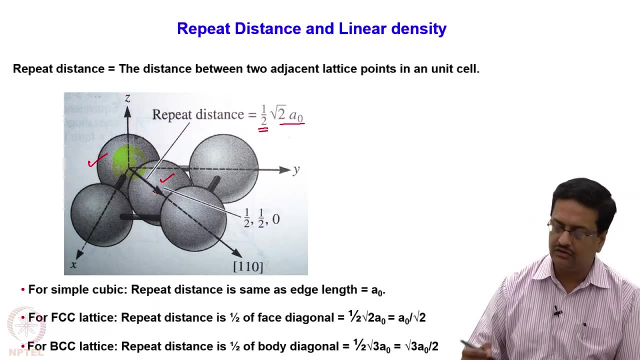 corner of the unit cell, one atom at the center of the face. So the face diagonal which is a distance called root 2 a, the repeat distance is half of that. So by moving along half of this diagonal we reach one particular lattice point. So for simple cubic that it is the repeat. 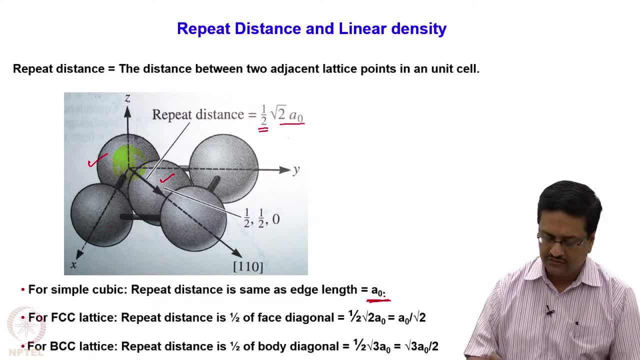 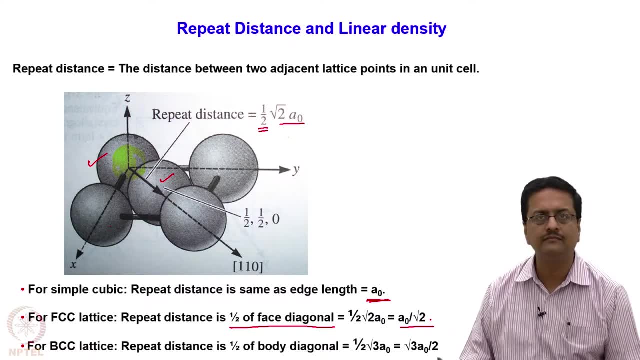 distance is same as a 0.. For face centered lattice it is half of the face diagonal, that is a 0 by root 2. and in case of body centered lattice the repeat distance is half of the body diagonal, which means half of root 3 by a 0. 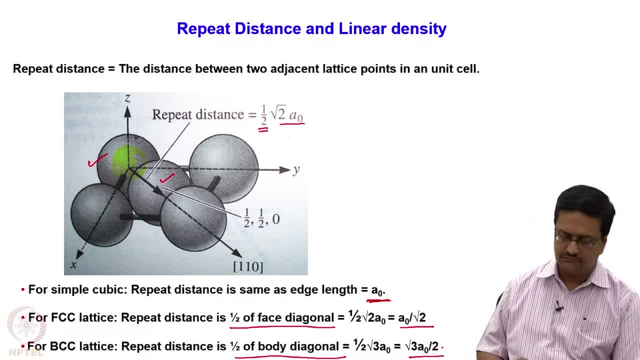 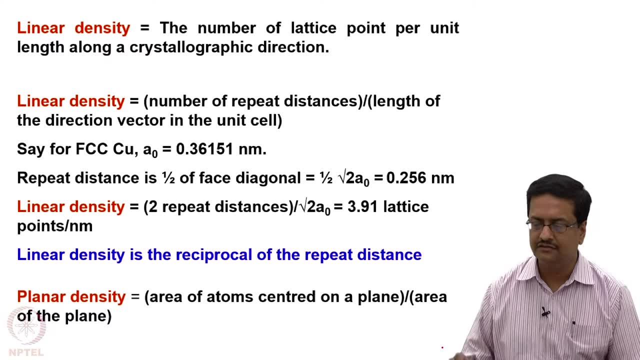 that is root, 3 by a, 0 by 2.. So the linear density is the number of lattice points per unit length along a crystallographic line direction. So linear density is basically the number of repeat distance per unit length of. 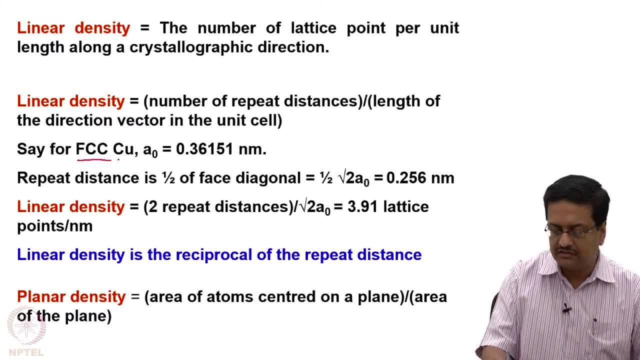 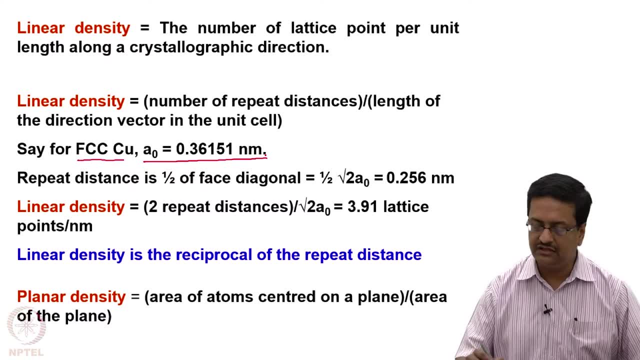 the direction vector. So for FCC copper, when the edge length is 0.36151 nanometer, the repeat distance is the phase diagonal. So we calculate it to be 0.256 nanometer. So the linear density is 2 repeat distances divided by the half of the body, divided by the 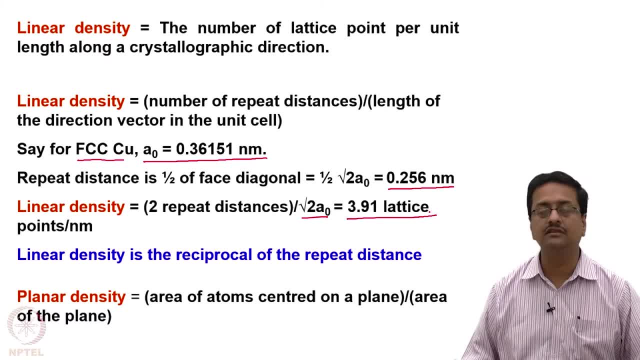 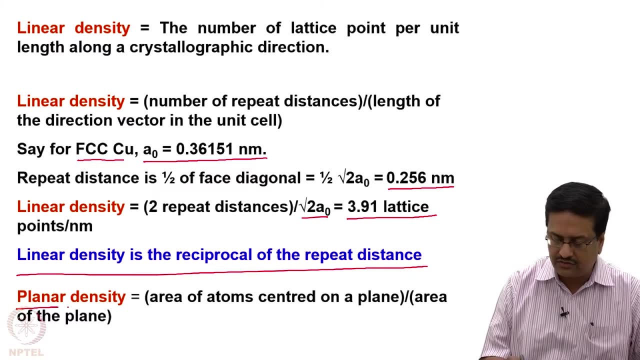 body diagonal, So 1.3.91 lattice points per nanometer. and linear density is the reciprocal of repeat distance. So similarly we can define another term called planar density, which means area of atom centered on a plane divided by the area of the plane. 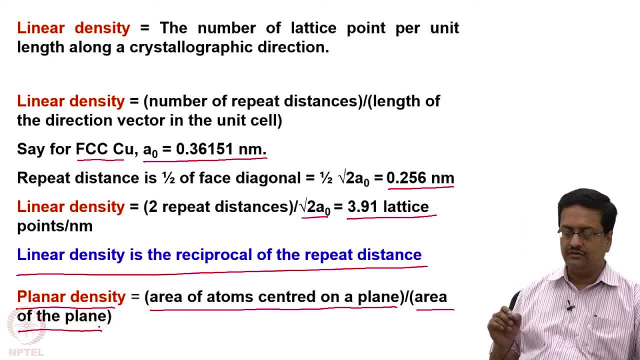 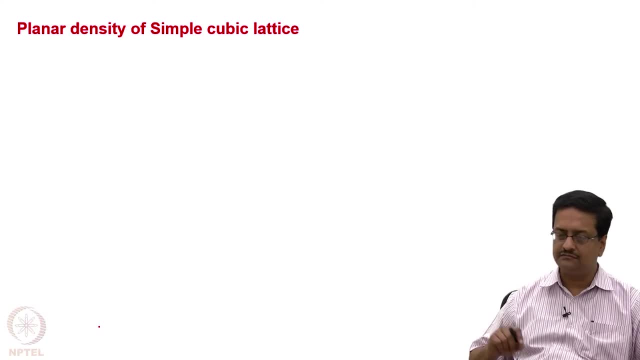 Because not all the planes will hold atoms, or not all the planes will hold the center of the atoms, and then the planar density of those planes will be different from the ones where you have large number of atoms. So in case of center of the plane, 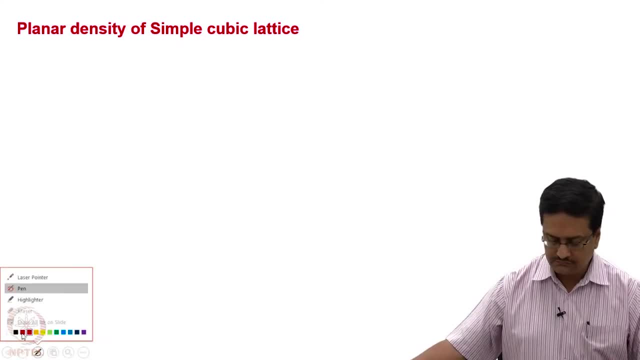 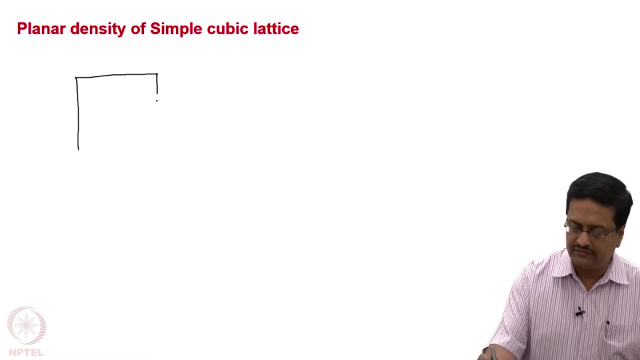 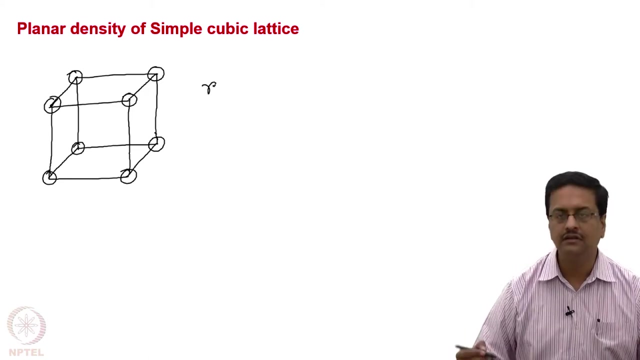 we just have a simple cubic lattice, which means it is a primitive lattice, and in that case what we have is that the 8 corners are occupied by 8 atoms or 8 lattice. So if we 8 lattice points and those 8 lattice points are such that the radius r is such that it touches, 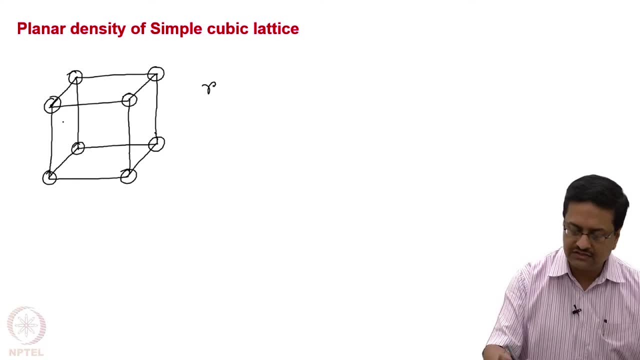 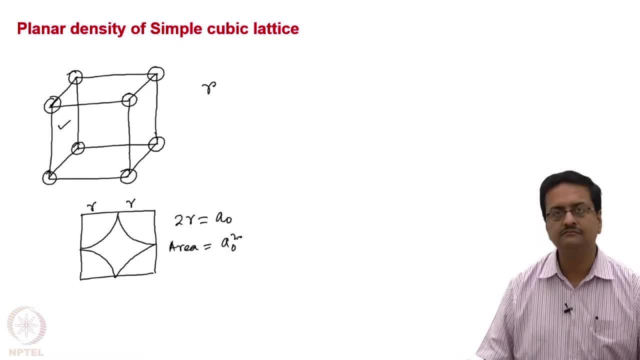 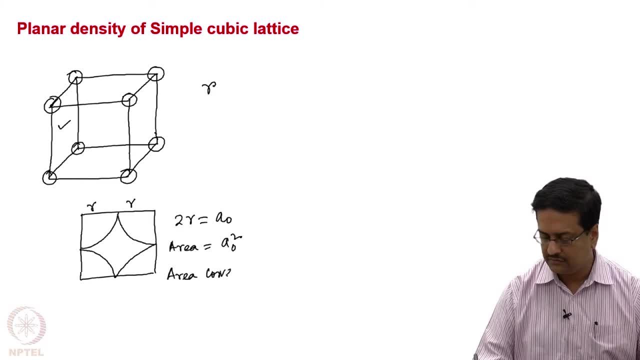 Area covered by the atoms is nothing but pi r square, because it is equivalent to one atom, because you have one-fourth, one-fourth, one-fourth, one-fourth, and we know r equal to a 0 by 2.. So here we write: pi a 0 by 2 square, that 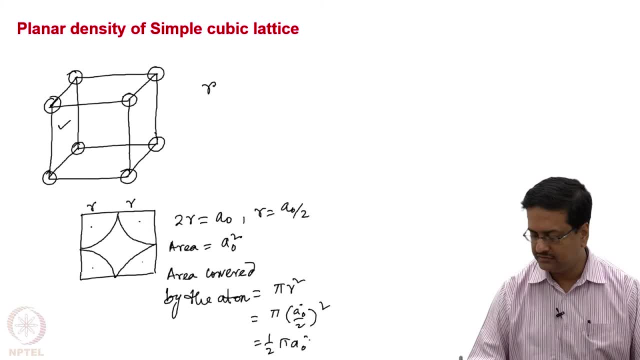 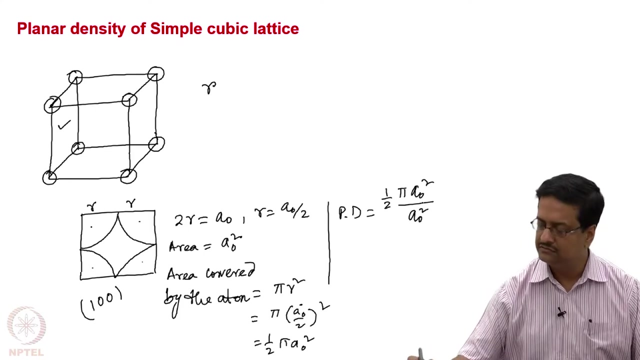 means half pi a 0 square. So the planar density for this 1, 0, 0 set of planes, which are the faces, would be the area covered by the atoms: half pi a 0 square divided by a 0 square. So this is nothing but equal to half pi. So now, if I want you to determine the planar density, 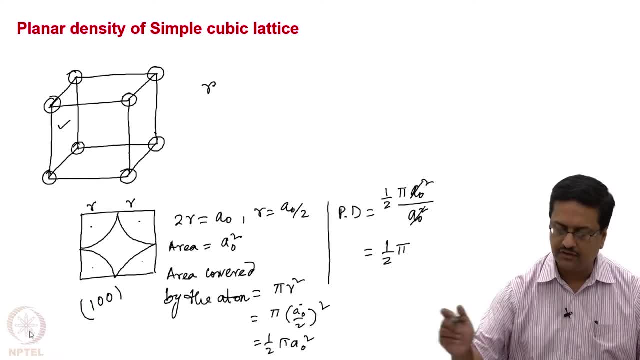 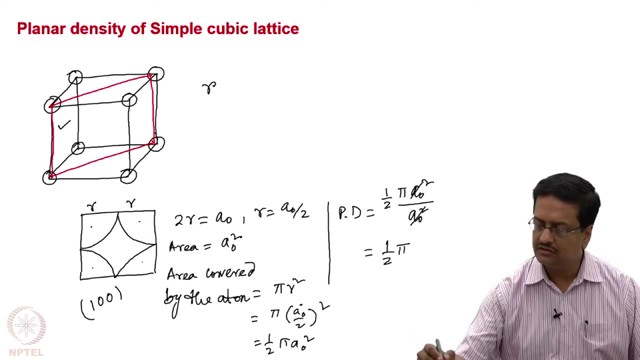 for the one-one-zero plane. how should we do that? we first should do the polynomial distribution of the plane as the set of planes. How should we perform it? the 1, 1, 0 plane, with the atoms placed on that, Along this edge, which is A. these two atoms are: 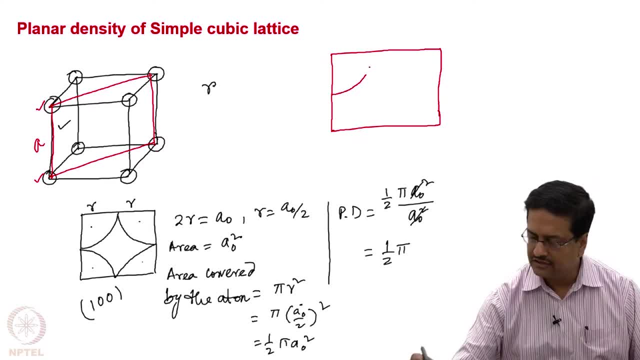 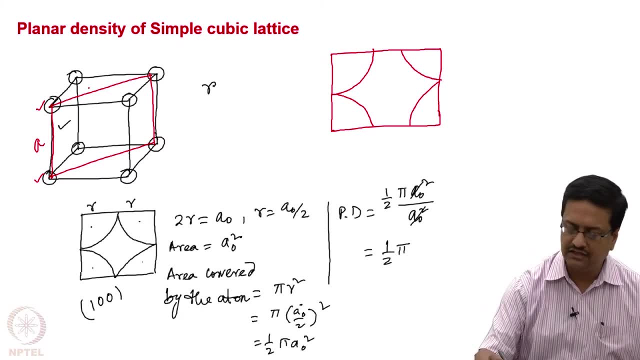 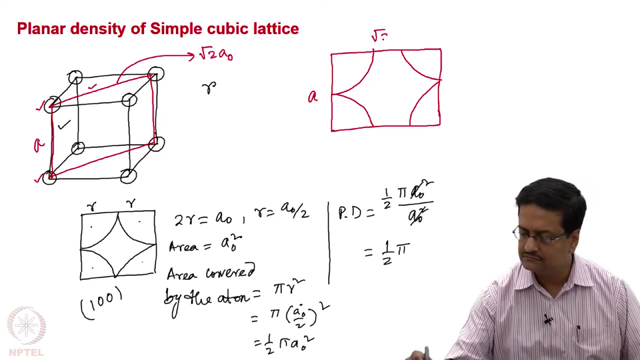 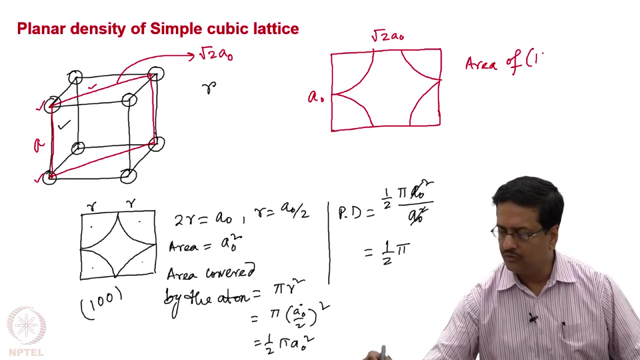 going to touch each other, So we write it like this: but along the face diagonal they do not touch, So there is a gap. Now what is the length of the face diagonal? The length of the face diagonal is root 2 A, or rather root 2 A- 0.. So what is the area of this face? Area of 1, 1, 0 set. of plane is 1 1 0.. So what is the area of this face? Area of 1 1 0 set of plane is 1 1 0.. So what is the area of 2 1 0 set of plane is 1 1 0.. So what is the area of this face? Area of 1 1 0 set. 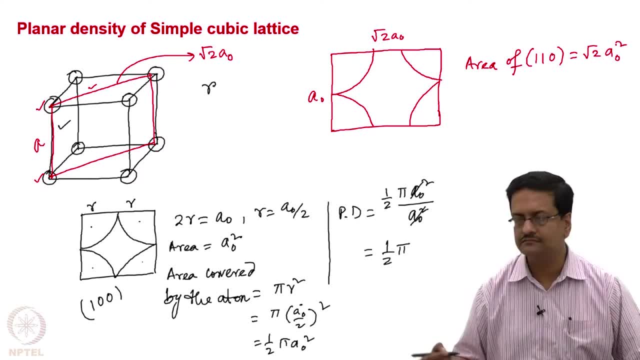 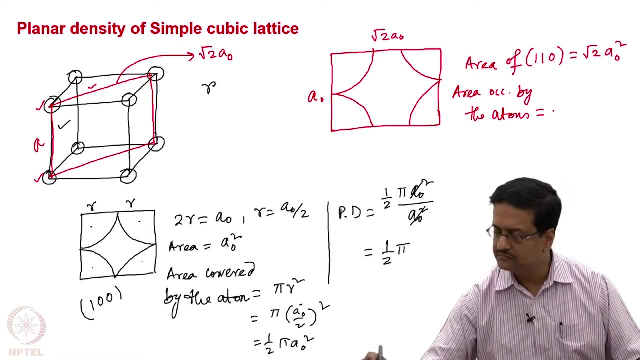 of plane is 1 1 0.. So what is the area of 2 1 0 sets of plane is 1: 1,. so what is root? 2 A 0 square Area occupied by the atoms is equal to, once again, pi R square, which is equal to pi A 0 by 2 square. 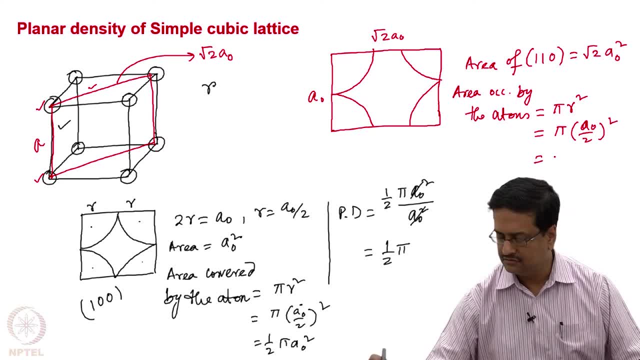 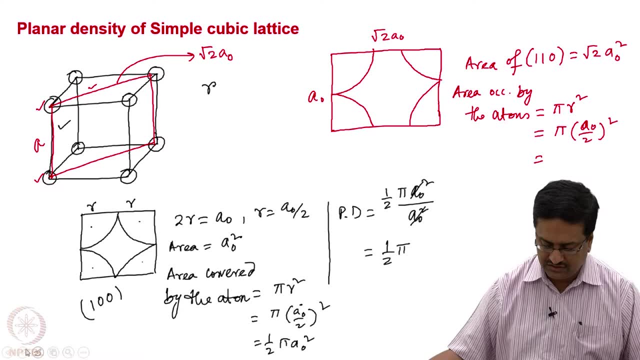 that is. One mistake here we have done is that this 2 is should be here 4. So one-fourth comes here. So now we do the same thing here as well. So one-fourth pi is century. So now we do the same thing here as well. So one-fourth pi is century Or two- kommer. 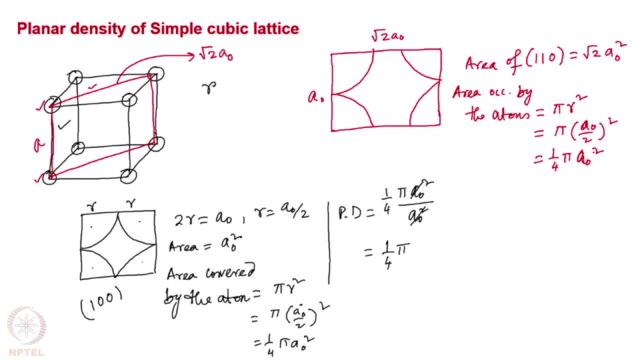 합니다 in an aspect ratio, So one-fourth à és snake Тут become two-fourth. So now we do the same thing here as well. so one-fourth coming here. So one-fourth pi 0 square. So the corresponding planar density will be one-fourth pi a 0 square divided by root. 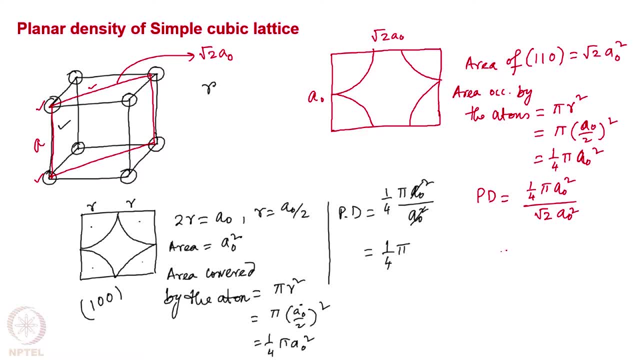 2 a 0 square, which means pi by 4 root 2.. So now we see that the planar density of 1, 0, 0 plane and 1 1, 0 plane are different. What will be the planar density of this particular? 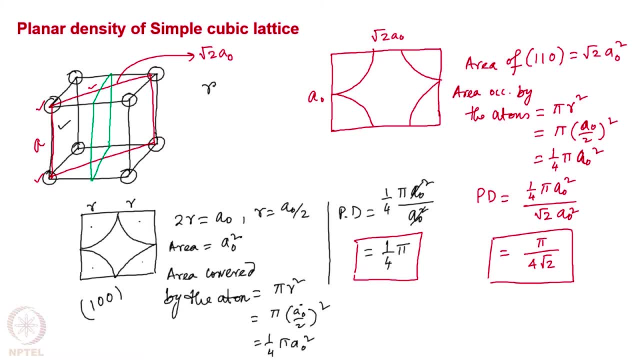 plane. What are the Miller indices for this plane? The Miller indices for that plane is: You see, here in this plane we do not have any atom centers located. That means no atom has contribution on this plane if we consider hard sphere. So the planar density is going. 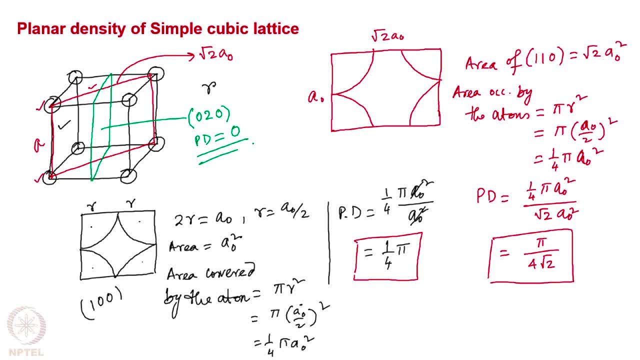 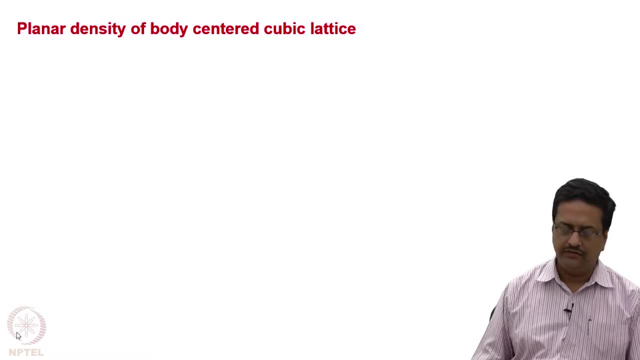 to be 0.. Now let us try to work out the planar density of body centered cubic lattice and we will try to see how the planar density changes for different planes like 100, 110 and 111 planes. So let us first draw the body centered lattice. As you know, the body centered 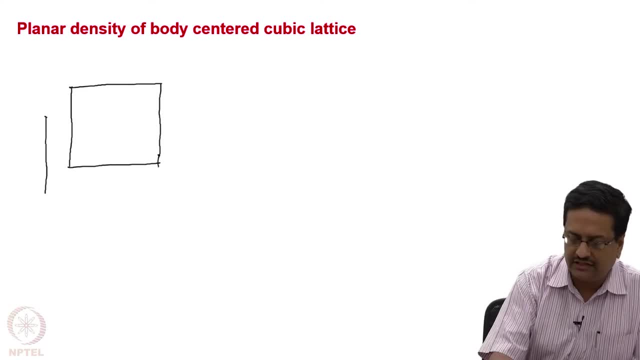 lattice has 8 lattice points at 8 corners and a lattice point at half half half. So we have atoms at 8 corners and at the center of the lattice. So in case of body centered lattice the close packed direction is at the center of the lattice. So that means the 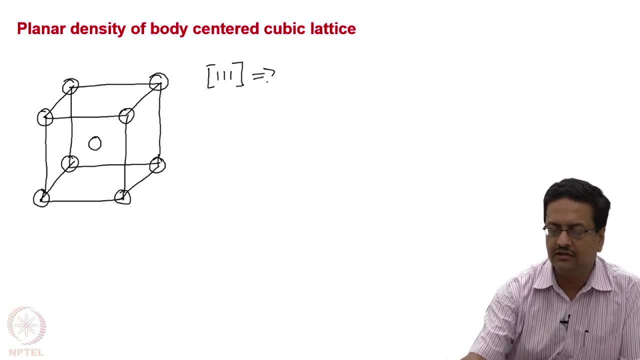 the 1, 1, 1 direction, that is the body diagonal. So if the edge length is a or a 0, the body diagonal is root 3, a- 0 and it is close packed along the body diagonal. So when we connect, 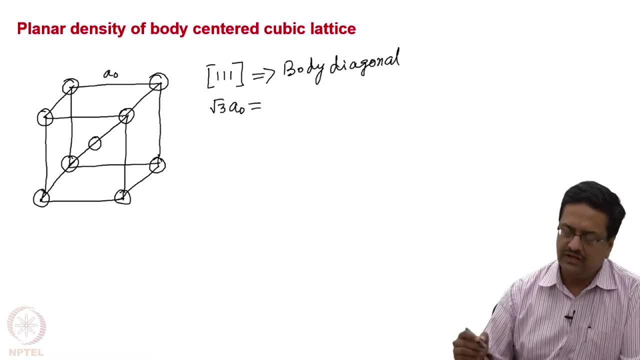 corner to corner, we pass through two atoms, So the diameter of two atoms is incorporated here. So the length in terms of atomic radius is 1, 1 r, which means r equal to root 3 by 4 a 0.. So now, with this in mind, let us start working. 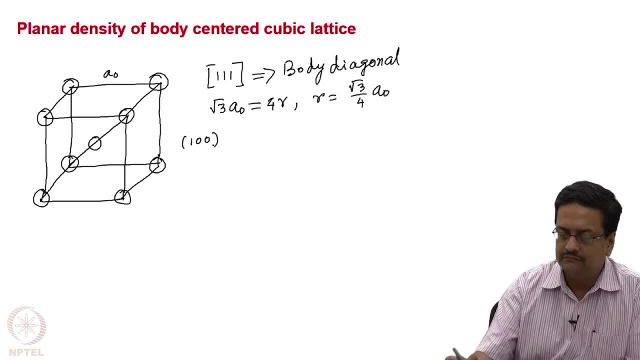 out the 1, 0, 0 plane. The 1, 0, 0 plane is the face, one of those six faces of a cube. and remember, since the body diagonal is the close back direction, the atoms do not touch along the face. The edge length of for the face is a 0. So the 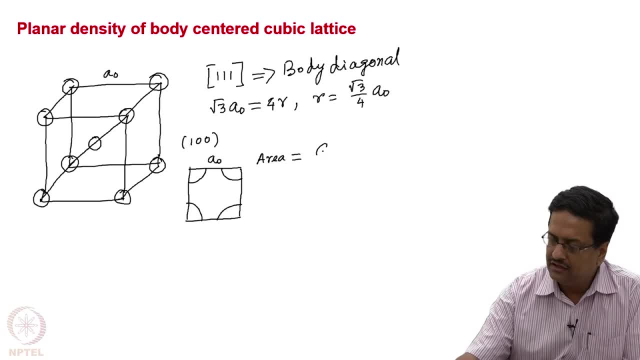 area of each face is a 0 square and the area covered by the atoms is nothing but pi r square, because one fourth, one fourth, one forth and one fourth gives you pi r square, which is equal to pi r square is root 3 a 0.. 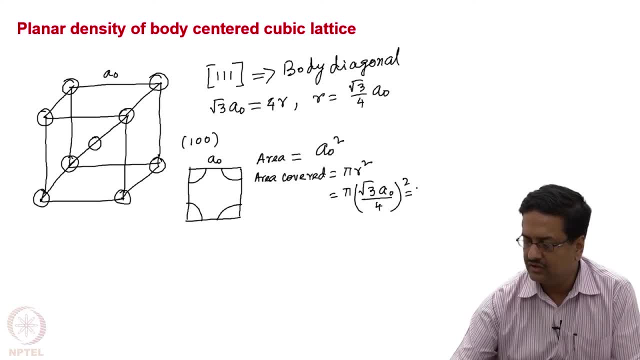 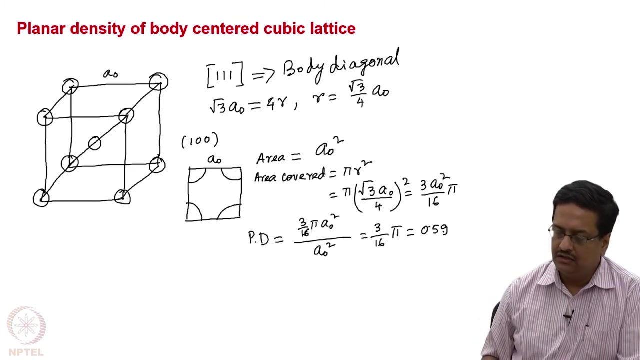 by 4 whole square, which is equal to 3 a 0 square by 16 pi. So now the corresponding planar density turns out to be 3 by 16 pi. a 0 square divided by a 0 square, which is equal to 3 by 16 pi, which is equal to 0.59.. Now, if we do it for the other plane, which 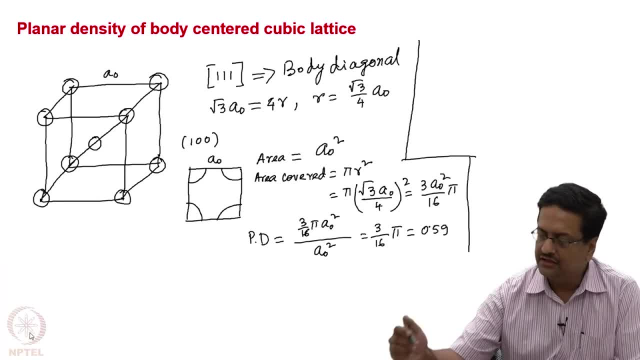 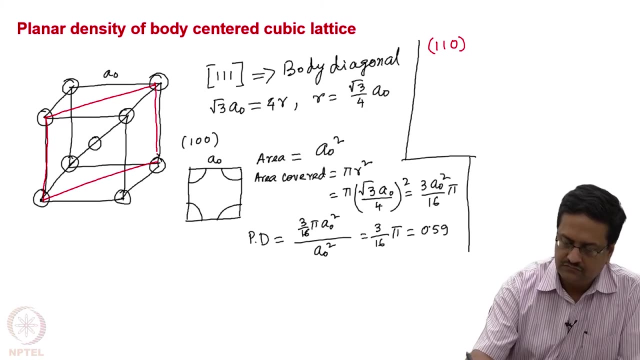 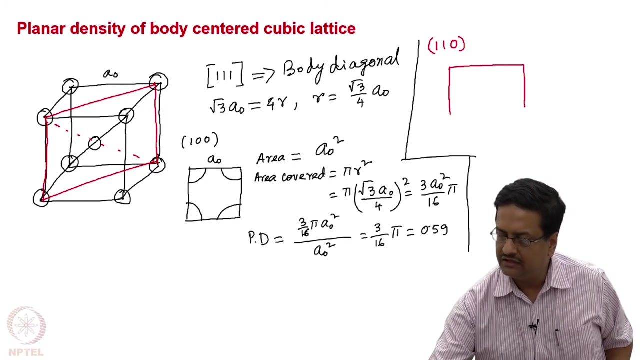 I told is the 1 1 0 plane. The 1 1 0 plane is the plane which I am drawing in red. So in this plane we have a body diagonal connecting the other corners. So if we try to draw the 1 1 0 plane in case of body centered cubic, 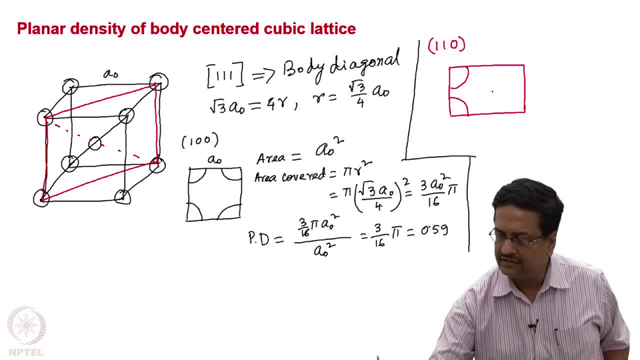 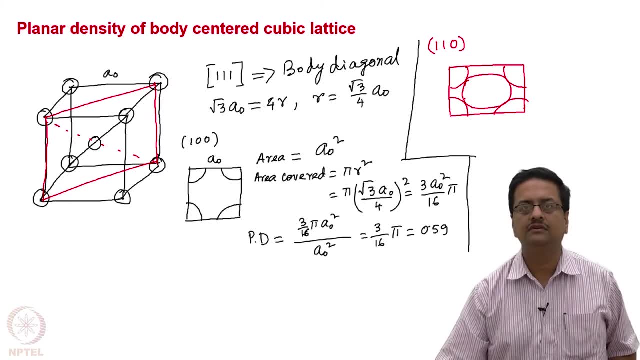 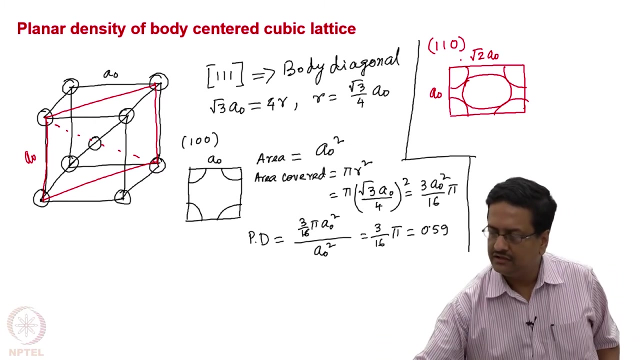 lattice we would have 4 atoms at 4 corners and the central atom would touch the 4 cornered atoms along the body. So the edge, one of the edge is a 0, which is this one, but the other edge is the face diagonal, which is root 2 a 0. So the area. 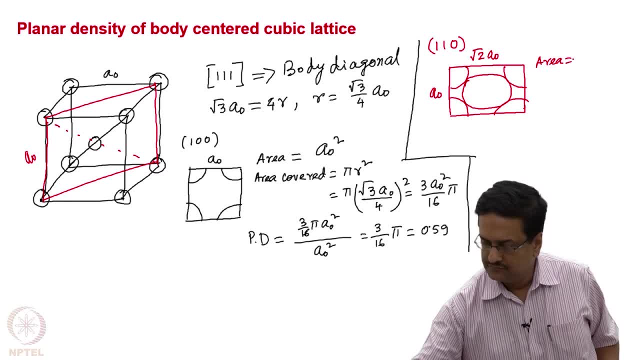 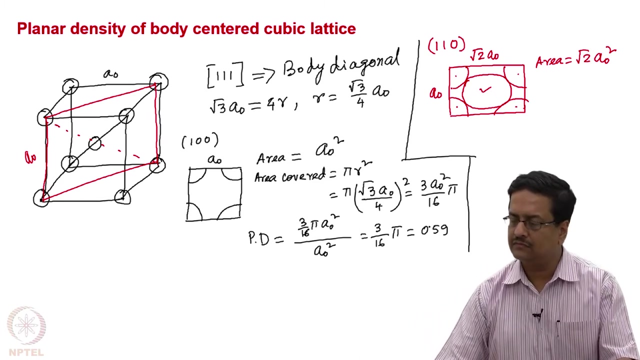 of the that it encompasses is root 2 a 0 square. Now inside this area you have 4 one-fourth portions of the atom and one full atom. That means total 2 atomic area is covered in this 1, 1, 0 plane of body centered lattice, So covering the entire body center lattice. So 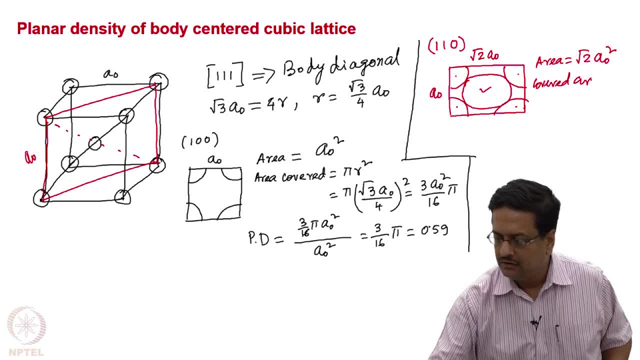 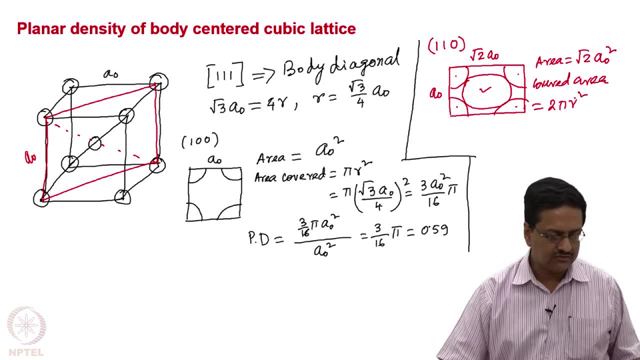 covered area is nothing but 2 pi r square. So this 2 pi r square can be written as 2 pi 3 a 0 square by 16, which means it is equal to 3 by 8 a 0 square. 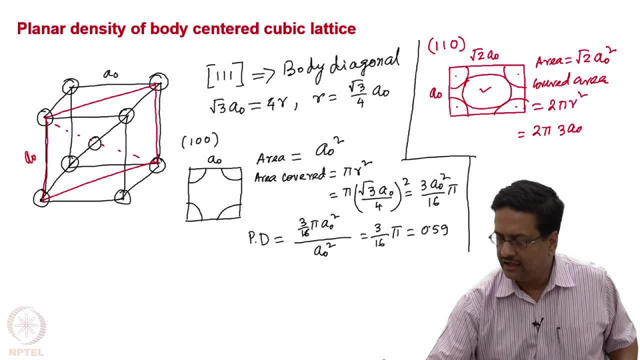 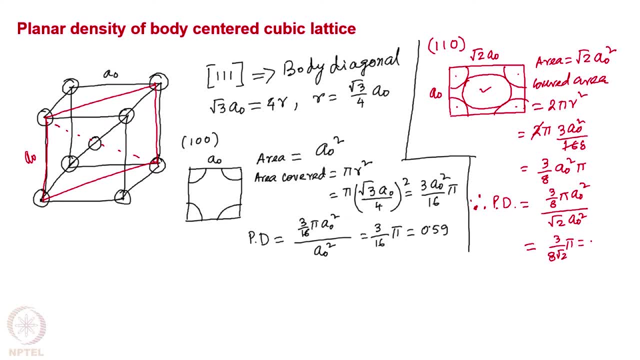 out to be 3 by 8 root 2 pi, which is equal to 0.89.. So now let us see what happens if we try to do the same for the plane 1 1 1.. Now you see that, interestingly, this 1 1 1 plane does not contain that point which is at half of half. 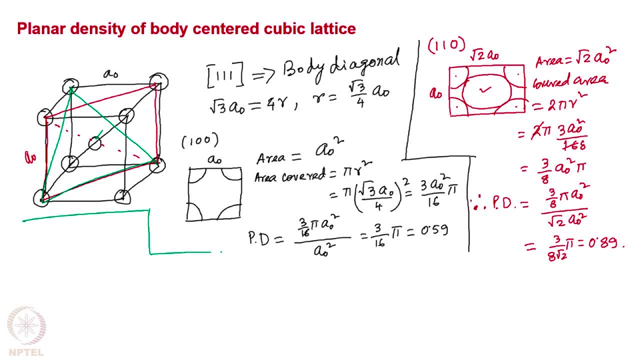 So the 1 1 1 plane, which is a triangular plane, should look like this, where we have three corners occupied by the atoms and the every side is corresponding to root 2 a. So the area under this triangle is nothing but root 2 a, square root 3 by 4, which means it is equal to. 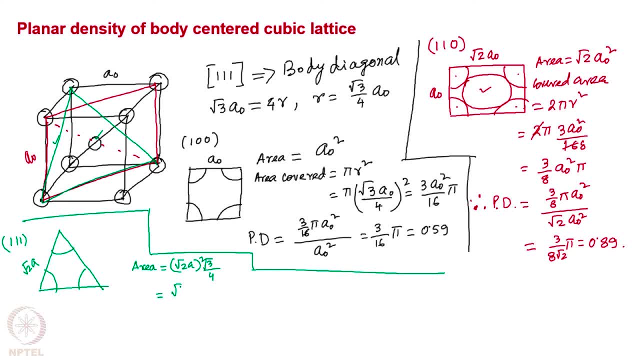 root 3 by 2 a 0 square. Now, the area covered is equal to one sixth, one sixth. one sixth, that means three parts of one sixth, means half pi r square. What is r? r is equal to root 3 by 4 a 0. 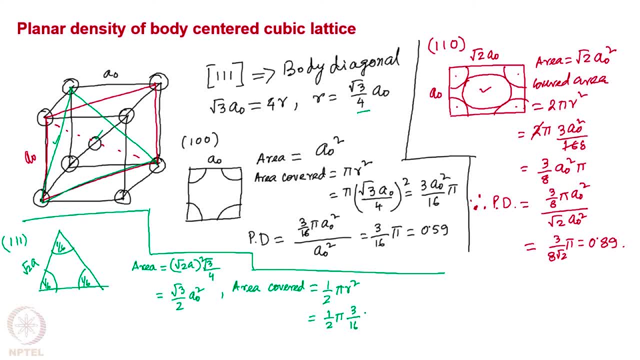 So a square is 3 by 16 a 0 square. That means the planar density is equal to the planar density is equal to 3 by 32 pi a 0 square divided by root: 3 by 2 a 0 square. 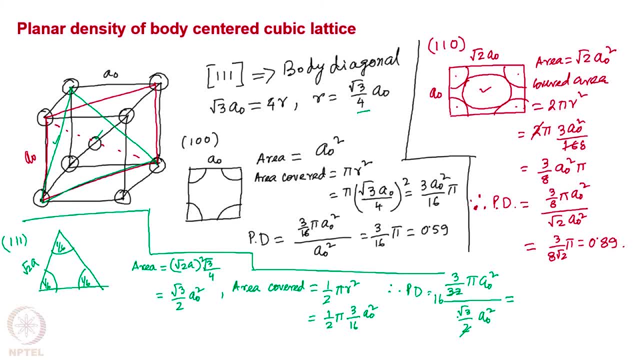 So you can work it out. So it is equal to root 3 by 16 pi, which means that the value turns out to be 0.34, a very small number. So this indicates that in case of body centered lattice, the plane 1 1- 0 has much higher planar density compared to. 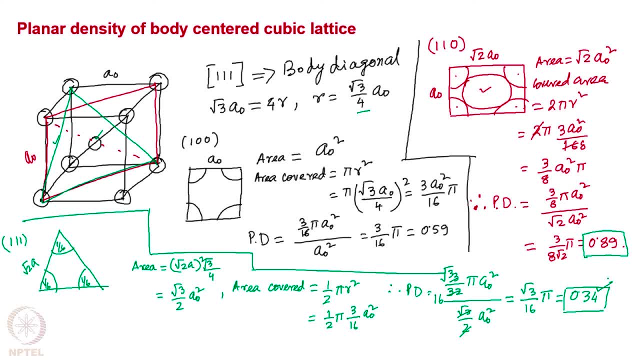 that of the 1, 1, 1 plane and the face. the plane which corresponds to the face, which is 1, 0, 0 plane, has an intermediate density. So in this lecture we have learned how to calculate the linear density and planar density. 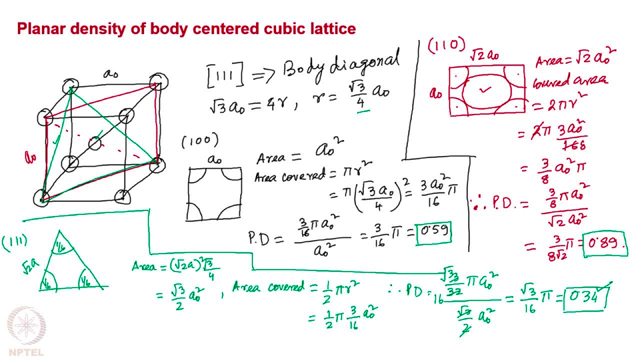 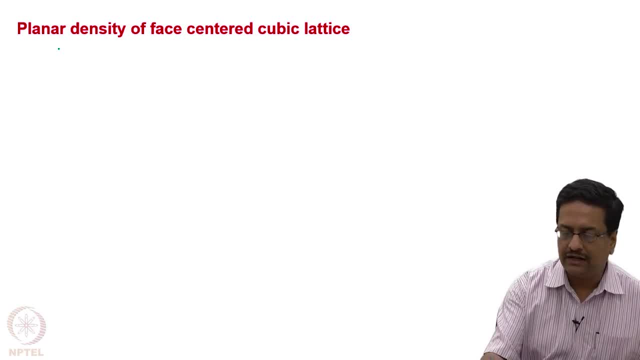 of different systems. So what I would like you to do yourself is to calculate the planar density of face centered cubic lattice for the planes 1 0 0, 1 1 0 and 1 1 1 and compare their values.